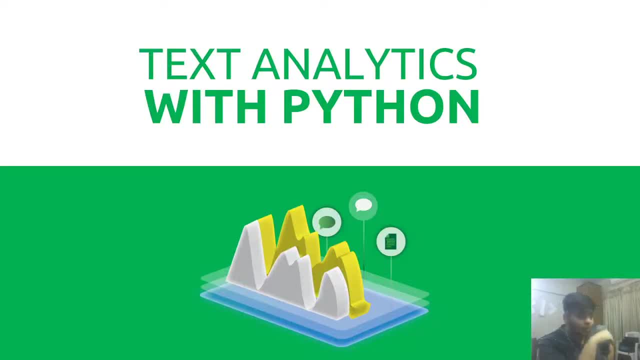 Hello, welcome back to another video, And in this video we are beginning a completely brand new course on text analytics with Python, And I'm so excited for this. I hope you are too, Because in this video we will be taking a deep dive into the basics of an NLP and how we can use one of the most strongest libraries, NLTK, in Python to process natural language. 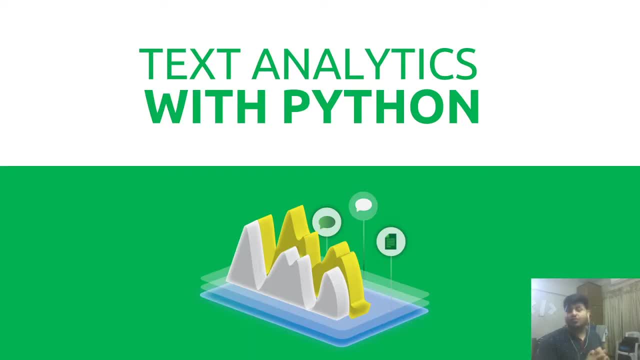 And, with that being said, we will also be using NLTK to implement one of the most famous and common applications in natural language processing, which is classification, summarization and so much more. So, to make this a little bit easier for you guys to understand, I've decided a plan of attack, And what exactly are we going to be doing in this whole series? 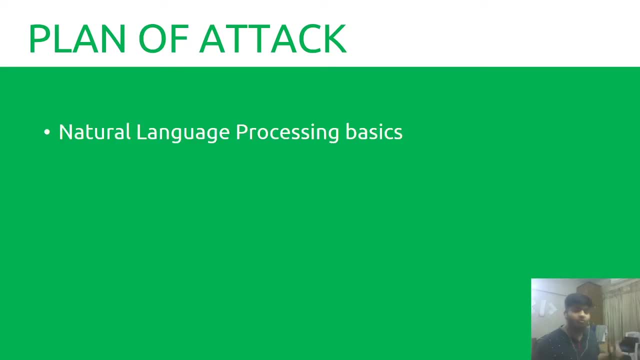 The first thing that we will be doing is natural language processing, the basics of natural language processing. We will be understanding the basics of natural language processing And the things that we need to know before we could dive into using Python's NLTK tool to implement the processing, or the basic processing, or basic functions to process natural language in Python. 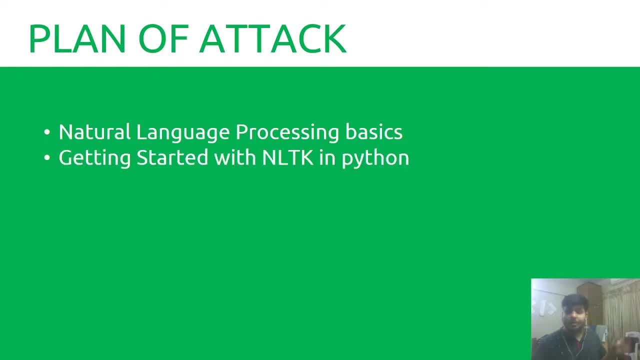 And, speaking of that, that's going to be the next part. We will be getting started with NLTK in Python And we will be learning the basics of Python, how we can implement some of the most common functions, such as word tokenization, lemmatization, removing stop words and stuff like that, in NLTK. And then we will be learning some of the most common functions, such as word tokenization, lemmatization, removing stop words and stuff like that in NLTK. And then we will be learning some of the most common functions, such as word tokenization, lemmatization, removing stop words and stuff like that in NLTK. And then, once we are done with that, we will be taking a look at how we can process natural language in Python with some of the advanced tools in NLTK. And then, once we are done with that, we will be taking a look at how we can process natural language in Python with some of the advanced tools in NLTK. And then, once we are done with that, we will be taking a look at how we can process natural language in Python with some of the advanced tools in NLTK. And then, once we are done with that, we will be taking a look at how we can process natural language in Python with some of the advanced tools in NLTK. 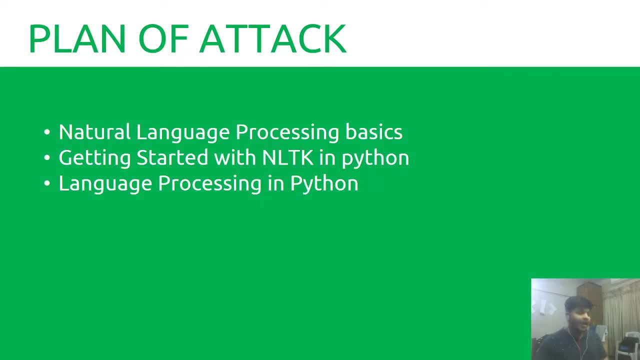 with some of the advanced tools in NLCK, and so by the end of this- these parts- you will be pretty good at processing natural language in Python. so, with that being done, we can get started with what the first application that we will be implementing with the text classification and since it's